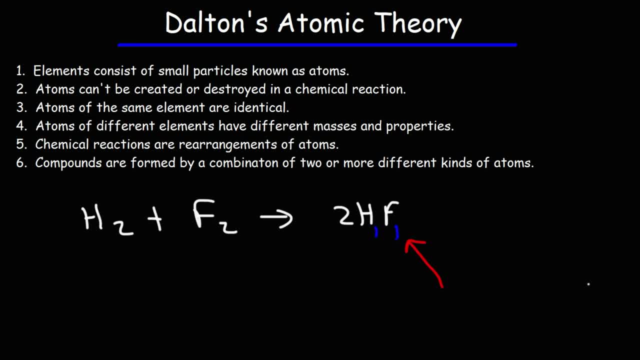 In this compound we have one atom of hydrogen and one fluorine atom. But the fluorine atoms, the hydrogen atoms, they were not destroyed in this reaction. They were simply rearranged into a new compound. So he also believed that compounds are formed by the combination of two or more different kinds of atoms. 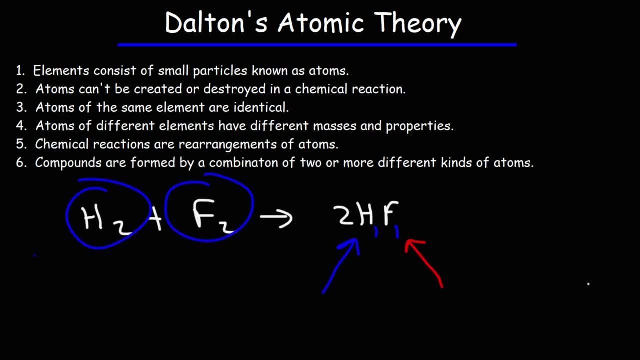 Here we have two different types of atoms and we were able to create a compound from that. Here's another example: Hydrogen gas reacts with nitrogen gas. Hydrogen gas reacts with hydrogen gas to produce ammonia. This reaction is associated with the Haber process. 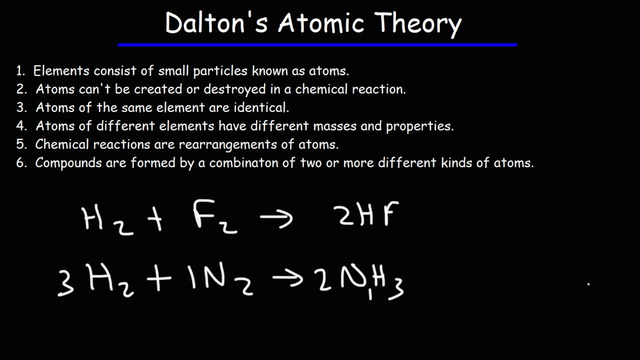 Ammonia is a compound that contains one atom of nitrogen and three atoms of hydrogen. So anytime you have a substance composed of different kinds of atoms, you have a compound. Now, some compounds have more than two different kinds of atoms. Baking soda, sodium bicarbonate, has four different kinds of atoms. 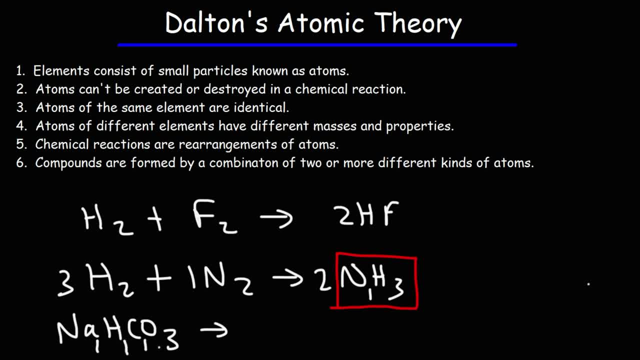 We have one sodium atom, one hydrogen atom, one carbon atom and three atoms of oxygen. So we have a total of six atoms in this compound, but four different types of atoms or four different elements. Now, John Dalton also believed that atoms of different elements have different masses. 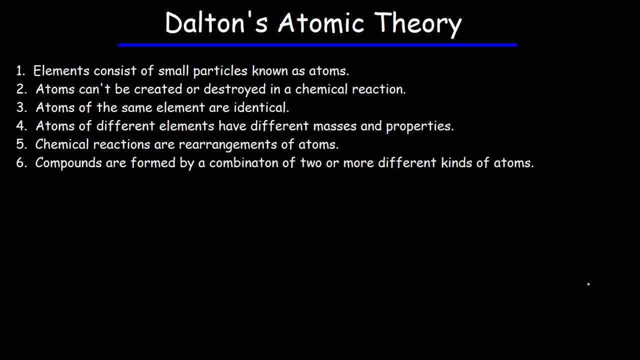 and different properties, And that makes sense. For instance, an atom of aluminum is going to behave differently than an atom of fluorine. Aluminum has an atomic number of 13.. Fluorine has an atomic number of 9.. The mass number of aluminum is 27, and for fluorine is 19.. 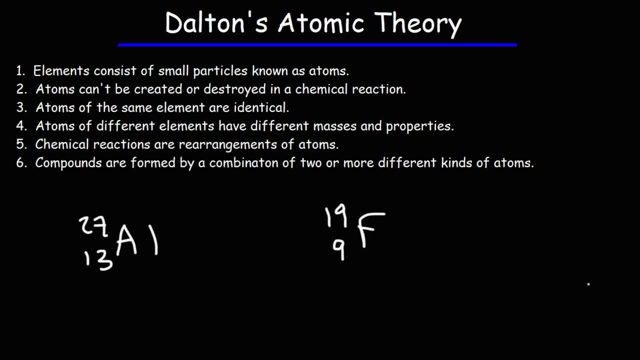 So because aluminum is a different element, it's going to have a different mass than fluorine. It will also have different chemicals. It's going to have different chemical properties than fluorine. Aluminum is a metal, Fluorine is a nonmetal. 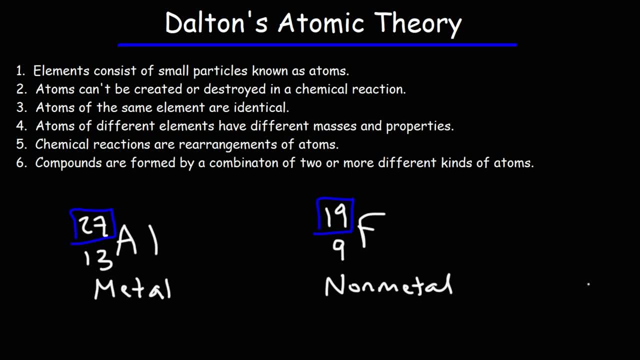 And, like other metals, aluminum wants to give away electrons. When it gives up its three valence electrons, it will form a cation. A cation is an ion with a positive charge. Fluorine being a nonmetal, it likes to acquire electrons. 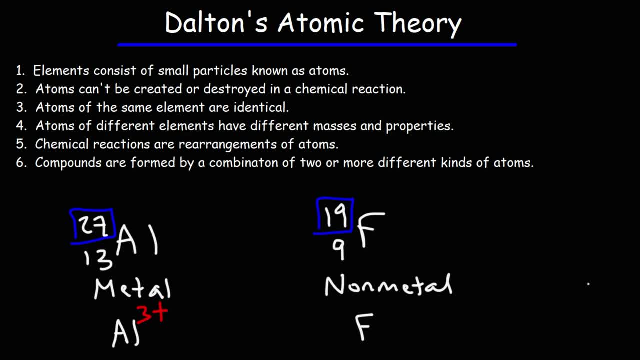 It's an oxidizing agent. When fluorine acquires one electron, it will form an ion with a negative charge, In this case fluoride. So metals like to give away their electrons to form positively charged cations. Nonmetals like to acquire electrons to form negatively charged anions. 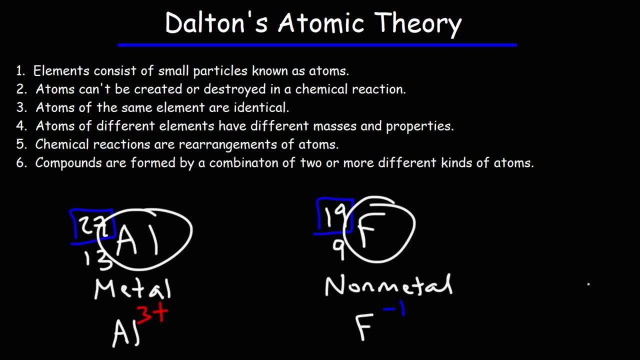 So these two elements, because they're different elements, their atoms have different chemical properties and different masses. Now, John Dalton also believed that atoms of the same element are identical And for the most part that's true, But you have to take into account isotopes. 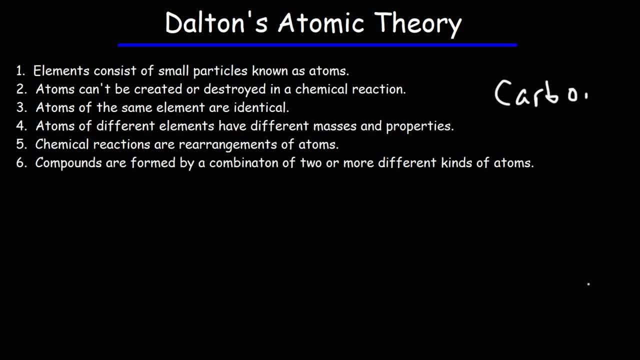 So, if we look at the element carbon, 99% of carbon is in the form of carbon-12.. The other 1% consists of carbon-13 and carbon-14.. So elemental carbon has different isotopes. Now these isotopes. 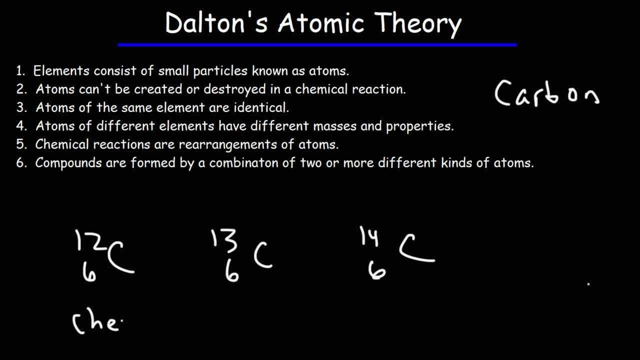 they have the same chemical properties But they differ in nuclear properties. So in a chemical reaction they will behave the same way, But in a nuclear reaction they will behave differently. Carbon-12 will react with oxygen to produce carbon dioxide- Carbon-14. 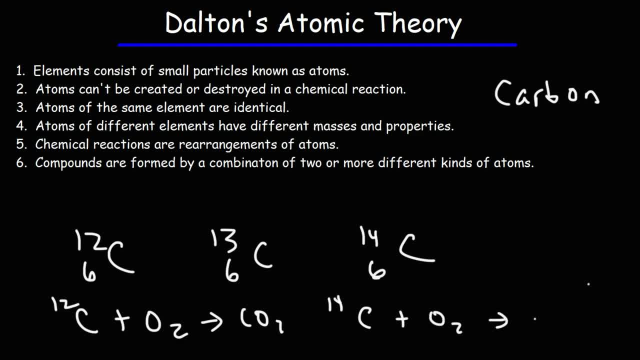 will even behave with oxygen, will also react with oxygen to produce carbon dioxide. So these atoms, even though they're different isotopes, they're still of the same element. They have the same chemical properties, but they do differ in their nuclear properties. 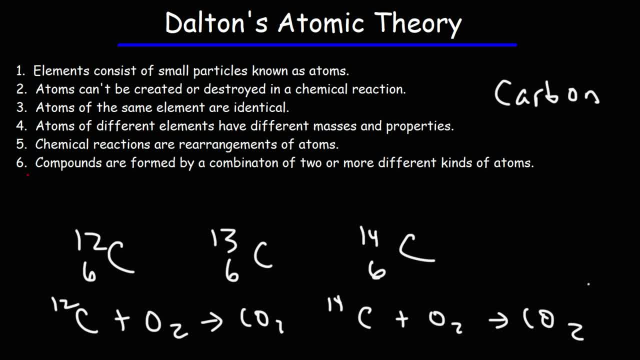 So that's the basic idea behind John Dalton's atomic theory. He believed that elements were composed of tiny particles known as atoms, and that these atoms are indivisible. He believed that they can't be created or destroyed in a chemical reaction and that atoms of the same element they're identical. 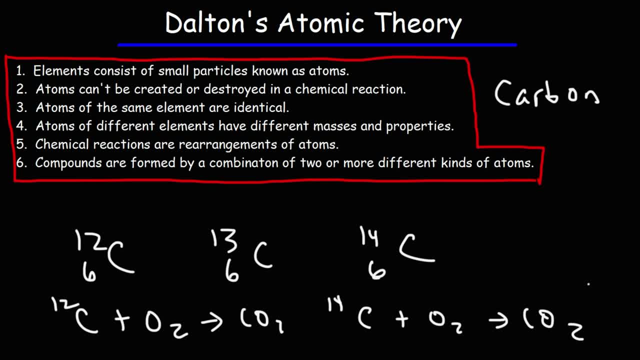 they have the same masses, they share the same chemical properties, and atoms of different elements have different masses and different chemical properties. He also believed that chemical reactions are simply rearrangements of atoms and that compounds are formed by a combination of two or more different kinds of atoms.